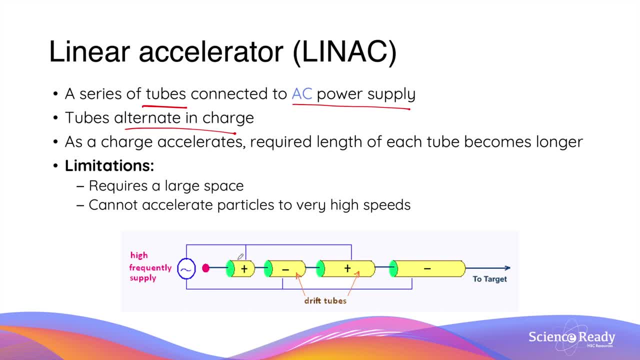 particle passes through the tubes, the AC power supply is able to alternate and change the charge. This means that the charges of the tube will accelerate the charged particle. So if we have a positive charged particle in the middle between the first and the second tube, this 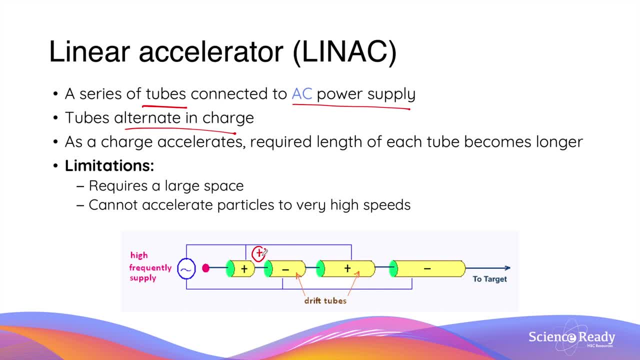 will be accelerated by the negative charge due to the attraction and be repelled by the first tube, which has the same charge. Therefore, it will increase in speed and accelerate forward. However, as the charge accelerates, its velocity gets higher and therefore it is able to cover. 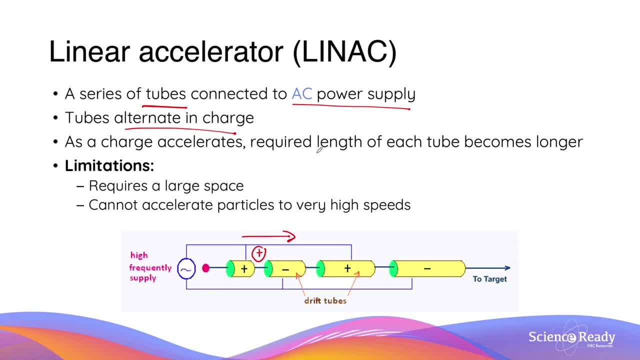 more distance in the same amount of time, So the required length of this tube becomes longer, As we want to make sure that the charge is able to experience the same amount of acceleration as is going through subsequent tubes. This requirement is actually one of the limitations of LINACs, Because this means to accelerate. 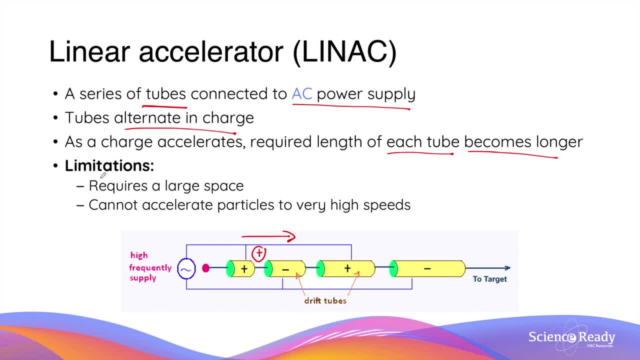 a particle to a very high speed, to what we want it to get to. it requires a very large space And, due to the space limitation, the linear accelerators, generally speaking, cannot accelerate particles to very high standards of speeds compared to the more modern forms. 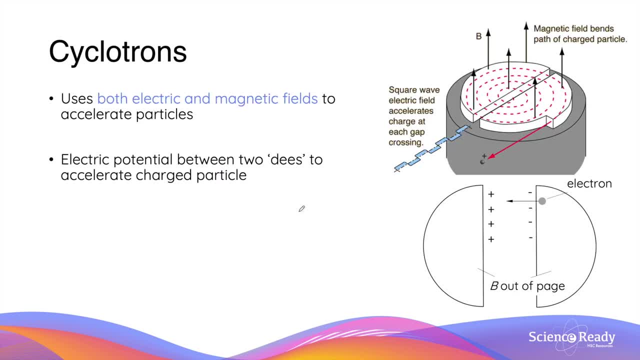 of particle accelerators. The cyclotrons are particle accelerators that use both electric fields as well as magnetic fields. This is one big difference between the LINACs and the cyclotrons, because the LINACs only use electric fields. The cyclotron consists of two main components: The first component, which consists of two. 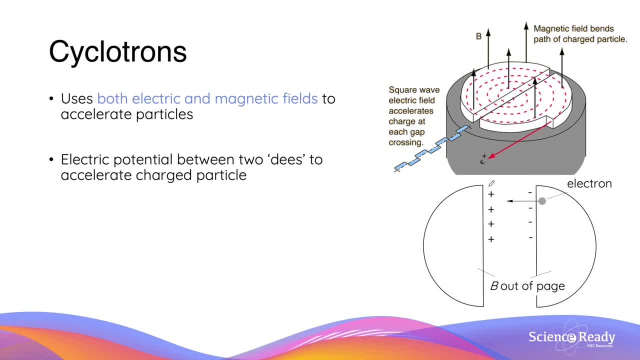 semicircles, and these are called Ds in a cyclotron. In the two semicircles we have an electric field created by a potential difference, And this potential difference is used to accelerate the charged particle as it is going across it. 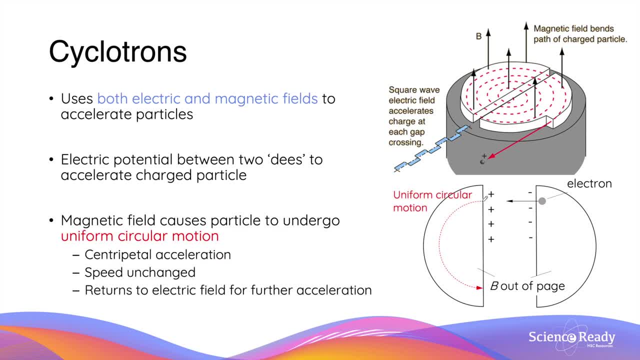 The magnetic field is located in the two semicircle Ds, such that when the charged particle crosses the electric field, it will undergo uniform circular motion inside the perpendicular magnetic field due to centripetal acceleration. It's important to note that the charged particle, although it does have a very large 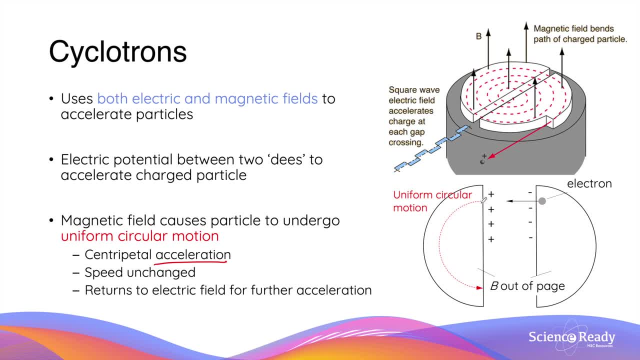 acceleration, its speed does not change. So once it completes the circular motion and returns to the electric field, its speed will remain unchanged. However, once it returns to the electric field, the charge across the electric field is then reversed to further accelerate the charged particle. 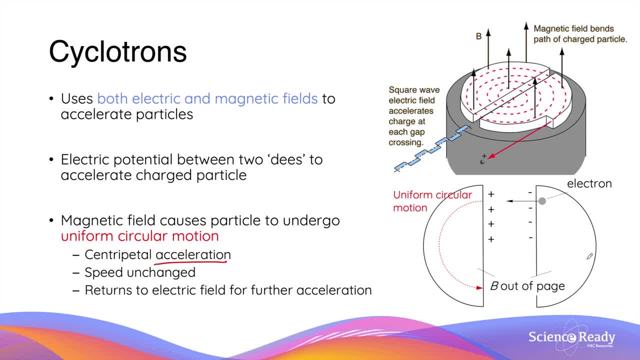 When the charged particle accelerates, it will then reach the other side of the cyclotron, whereby there will be another perpendicular magnetic field To facilitate another round of circular motion. This process will then repeat, and every time the particle goes around a circle, its speed. 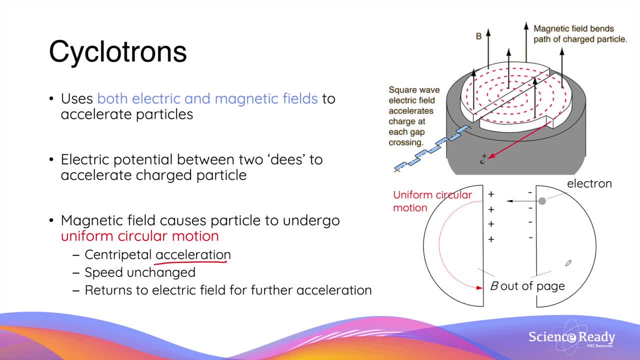 will increase in a consistent manner. Now you can imagine, a major advantage of the cyclotron over the linear accelerators is that the acceleration of these particles is facilitated in a cyclic manner. Therefore, the size of the cyclotron can be made much smaller compared to the linear accelerators. 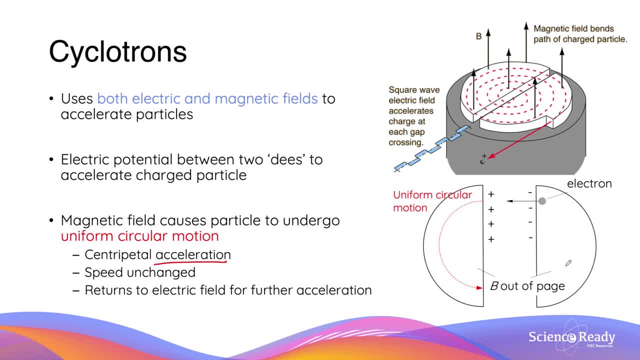 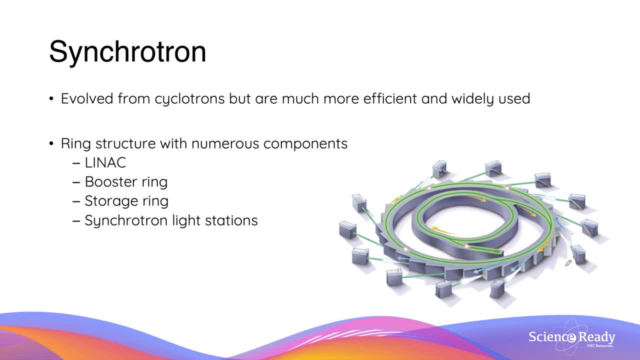 This is why cyclotrons don't move Cyclotrons. generally speaking, they can accelerate particles to much higher speeds compared to the LINACs can. The synchrotrons are the mainstay of particle accelerators we use in modern physics. 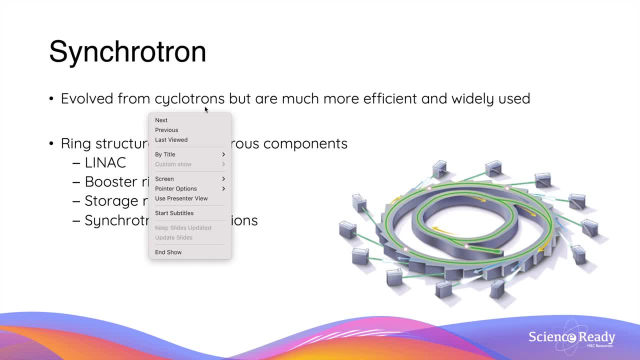 And these accelerators evolved from the cyclotrons, but these are more efficient and more widely used nowadays. The synchrotron has a very complex structure. It's got numerous components. It's made of a LINAC, a booster ring, a storage ring and what we call synchrotron. 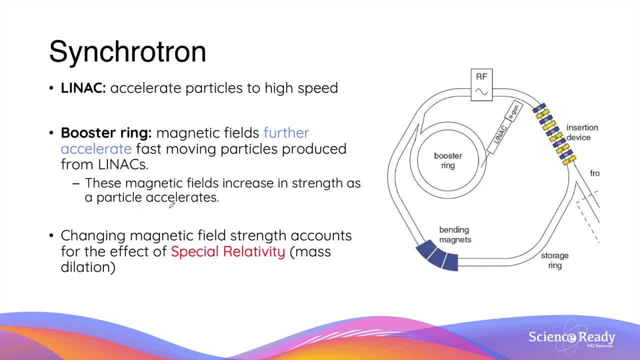 light stations. We'll talk about these components individually. This is a bird's eye view of a synchrotron. In the middle of the synchrotron we have a relatively small LINAC, which is a linear accelerator. This is used to accelerate particles from rest to very high speeds. 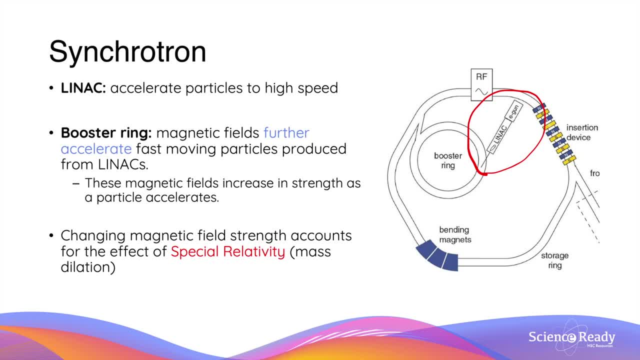 And once the LINAC accelerates the particles to the speed that we want it to, this enters the booster ring, in which the particles are further accelerated by magnetic fields to the speed that it will launch. The reason why this is known as a synchrotron is because the magnetic field strength of 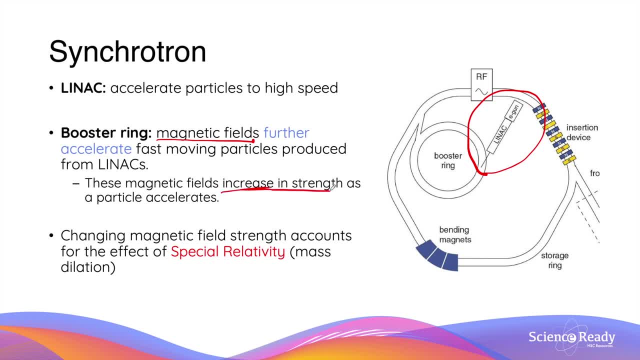 the magnets in the booster ring can increase in strength accordingly as the particle accelerates. Now remember that the radius of circular motion depends on mass times, velocity divided by charge and magnetic field strength. As the velocity of the particle increases, The synchrotron is able to ramp up. 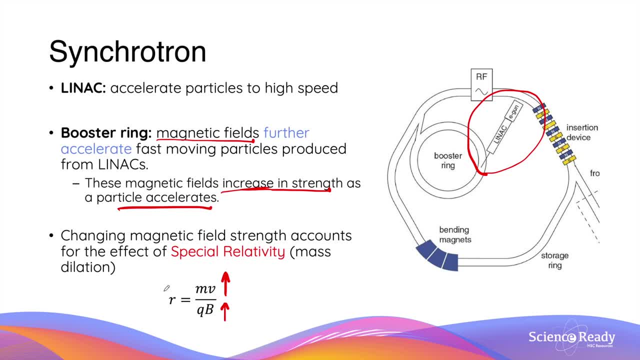 its magnetic field strength, such that the radius of the circular motion remains the same and, as such, the particle is able to go around and round the booster ring many, many, many times per second and reach to a high speed in a very short duration of time. What's also very fascinating about synchrotrons? 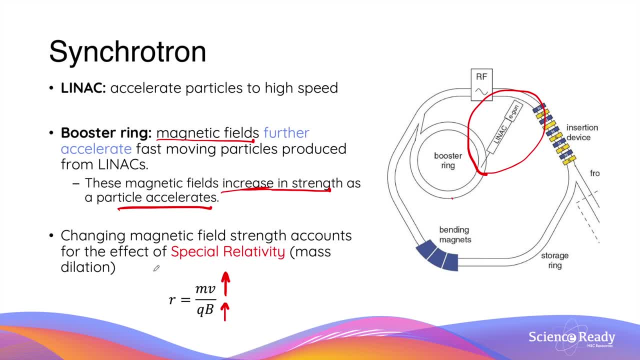 is that as the particle reaches a very high speed, eventually the effect of special relativity will kick in, namely mass dilation. Recall that the mass of a particle will increase drastically when its speed reaches a fraction of the speed of light. The change in magnetic field in the synchrotron also. 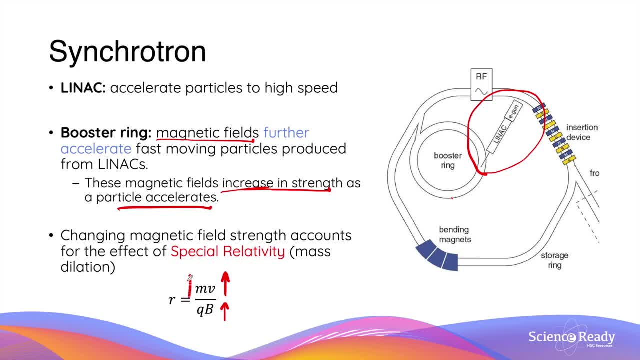 accounts for this effect, such that as the mass of the particle increases, the magnetic field also increases the more, to account for not only the velocity but also the increase in mass. In essence, in a synchrotron, the strength of the, the magnetic field, is adjusted so that it is in sync with the velocity and the 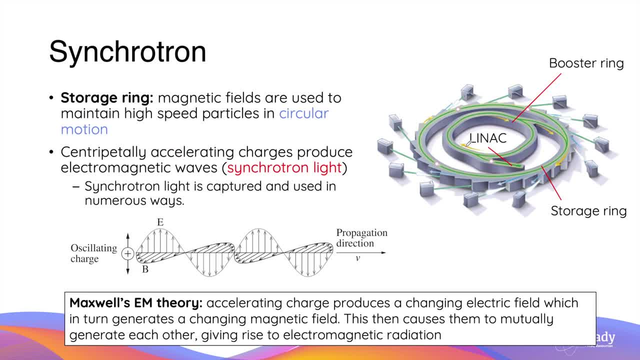 mass of the charged particle. When the velocity goes around the booster ring, eventually it will reach the speed that we want it to. The particles which reach the desired speed is then ejected into the outer ring of the synchrotron, known as the storage ring. In the storage ring, the high speed particles are maintained. 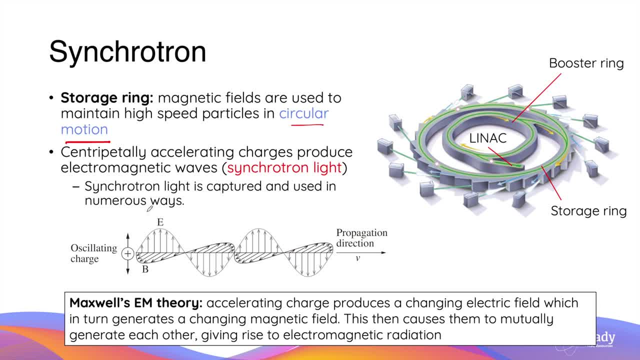 at the speed are in circular motion, and when they are in circular motion they will experience centripetal acceleration. Recall that in Maxwell's electromagnetic theory he postulated that when we have an accelerating charge it will produce a magnetic field as well as an electric field. and if this accelerating charge is 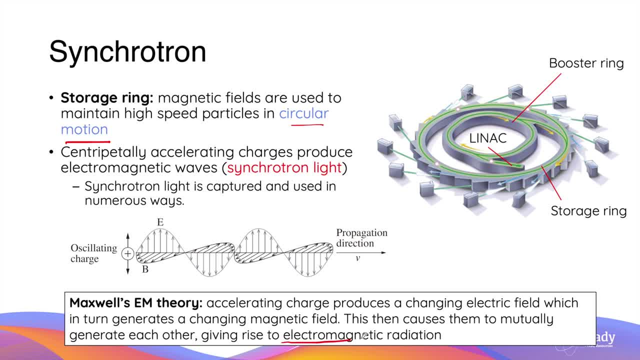 propagating. it will then give rise to electromagnetic radiation. So when a high-speed charged particle is undergoing centripetal acceleration, ie circular motion, it will produce EMR, and this EMR is called synchrotron light. The synchrotron light is then captured by 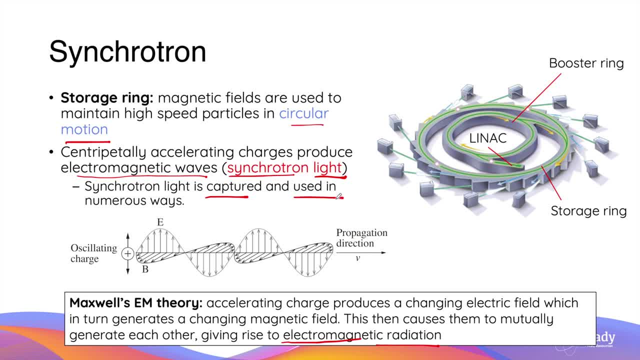 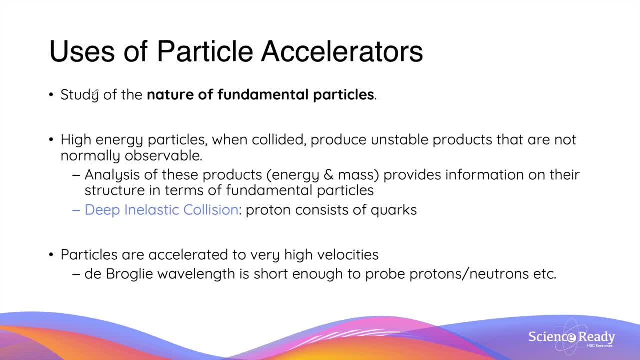 various stations around the synchrotron and used in different applications. There are many applications of particle accelerators. Primarily in physics, particle accelerators are used to study the nature of fundamental particles. When particles reach high speed, they will possess very high amounts of kinetic energy, and these high energy 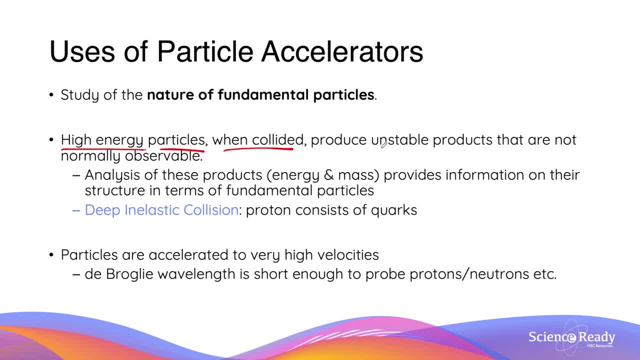 particles, when collided with one another, can produce unstable products that we do not normally see and observe in normal situations, And by analysing these products, for example the energy and mass, this will give us information on the structure in terms of the elementary or fundamental particles that we learnt about in the standard model of matter, To give you. 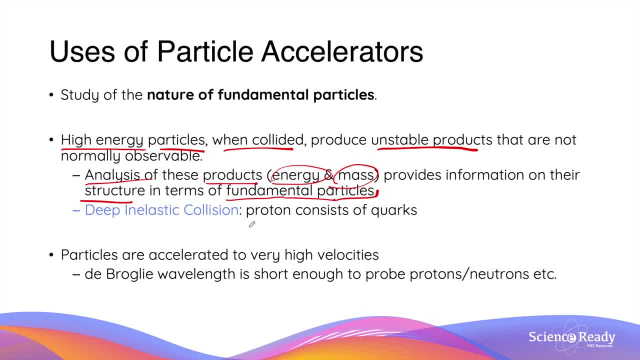 an example, particle accelerators were originally used to collide an electron with a proton in an experiment called the deep inelastic scattering or collision, And this collision showed that protons were made of smaller particles called quarks. More recently, particles that were accelerated by high velocities were also shown to exhibit wave-like properties, and this confirms. 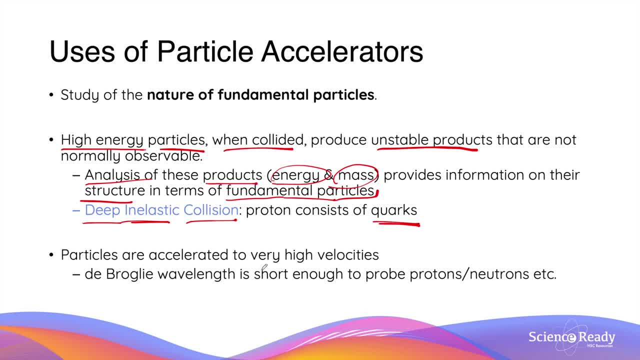 the matter and wave duality of high-speed masses. The de Broglie wavelengths were, in fact, short enough to probe protons and neutrons by producing images as a result of diffraction and interference, A very similar principle that was used in the investigation of the nickel crystal structure by Davison and Germer. 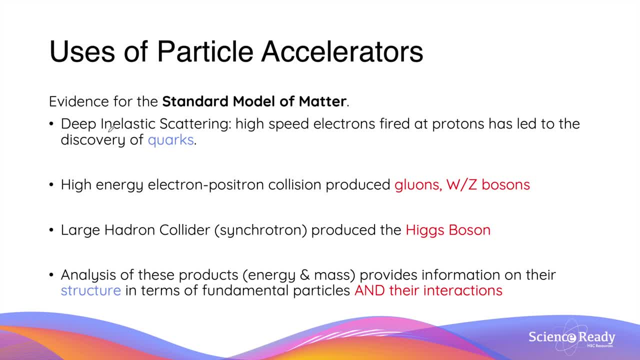 In addition to the discovery of quarks, particle accelerators also provided evidence for other particles. part of the model, The high energy collision between electrons and positrons produced gluons, as well as the W and Z bosons that mediates the weak forces. 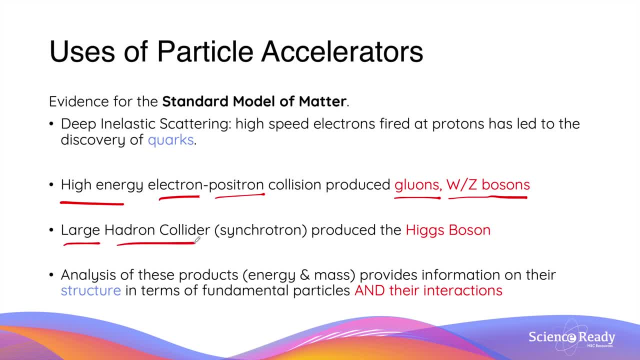 A particular particle accelerator called the Large Hadron Collider, which is a synchrotron, produced the Higgs Boson in 2013.. So, by analysing these products, not only are we able to obtain information on the structure of fundamental particles, we are also able to study the forces and the interactions between 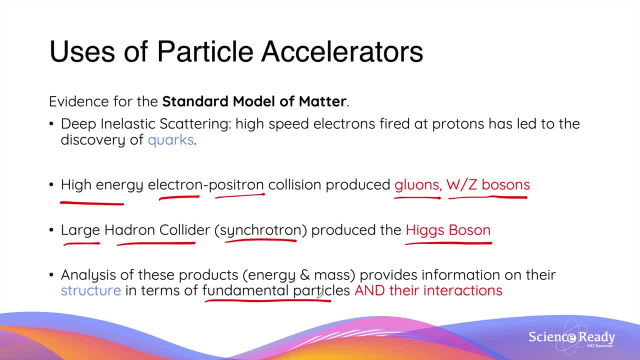 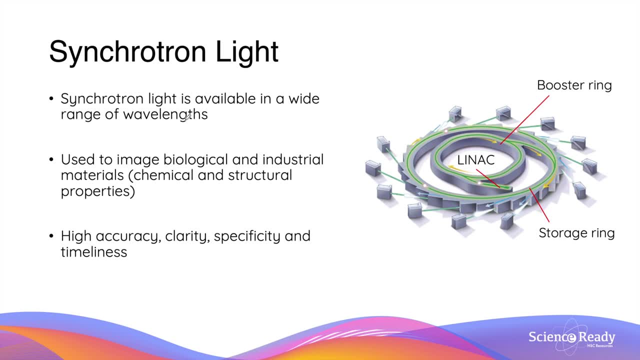 these particles, In this case by discovering the various bosons in the standard model of matter. As I mentioned earlier, when the particles enter the storage ring on the outside of the synchrotron, they will produce EMR, that's known as synchrotron light. 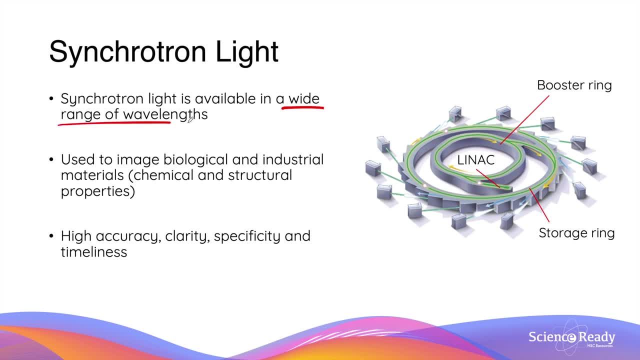 The synchrotron light is available in a wide range of different wavelengths. Remember that the wavelength or frequency of the radiation depends on the acceleration of the charge. So the beauty of using a synchrotron to produce the synchrotron light is that we can control. 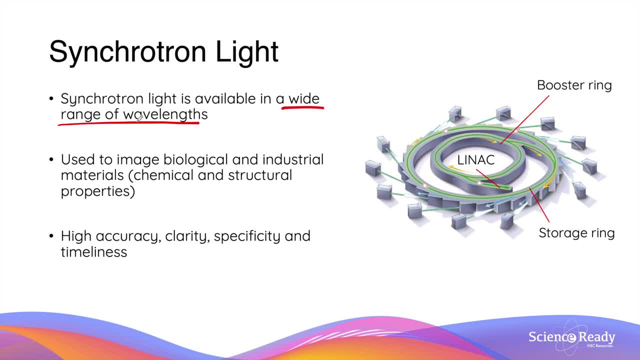 the exact wavelength of the synchrotron light that's being produced by the charge. Synchrotron light can be used to image biological and industrial materials to identify and analyze the chemical and structural properties. In general, the advantages of synchrotron light is that they are highly accurate, very 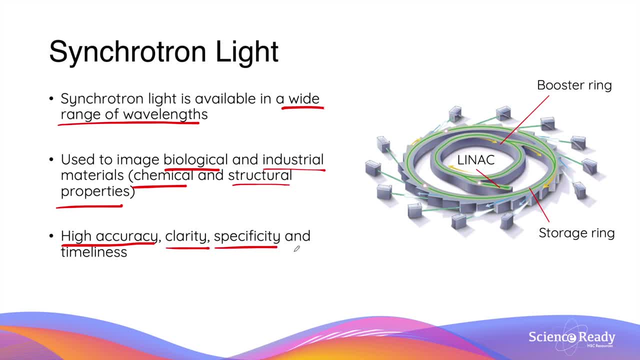 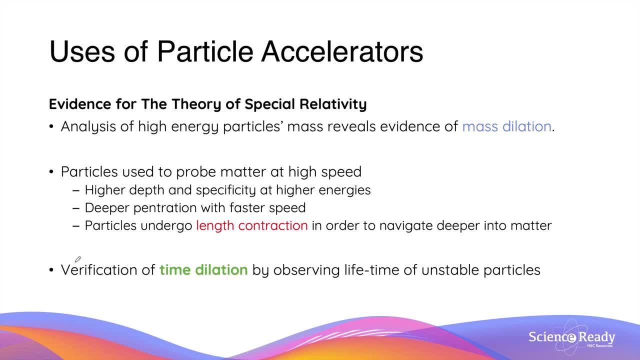 very high in clarity and specificity, and they can be produced in a very short time. Now, besides the standard model of matter, particle accelerators also provided evidence to support the theory of special relativity. We talked about how, by analyzing the high energy and the mass of particles, we can understand. 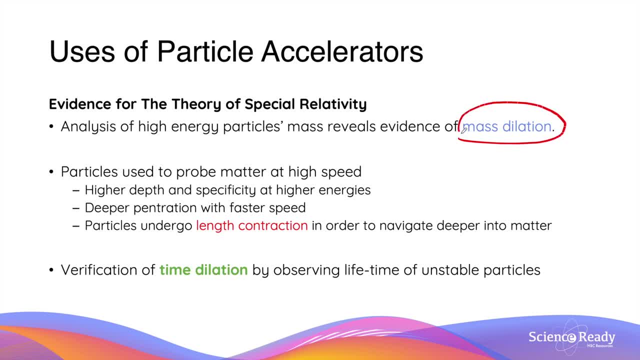 them. but this has also revealed evidence of mass dilation, as we are able to show that particles do in fact gain mass as they reach speeds near the speed of light. High speed particles are also used to probe matter. This has allowed us to understand the theory of special relativity. 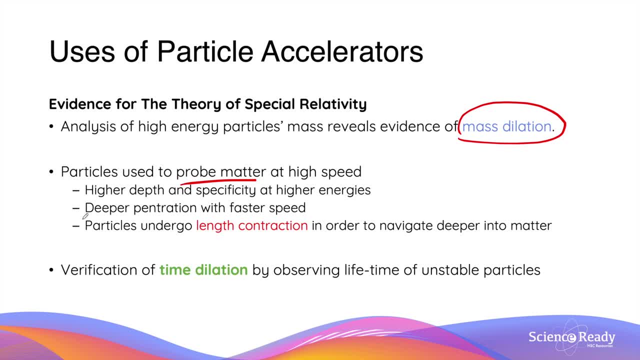 Particles are able to achieve deeper penetration into materials the faster they are travelling. This is an indirect piece of evidence for length contraction, which is a consequence of special relativity. This is because particles, when they are travelling faster, they will undergo length contraction. 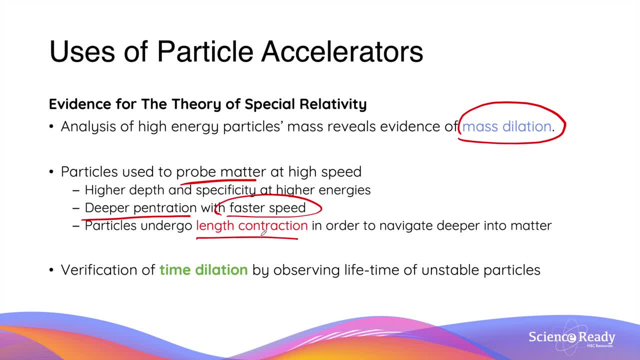 to achieve a smaller dimension, And when the particles are smaller in dimension, they can then navigate deeper into the matter due to smaller physical constraints. Furthermore, particle accelerators, through producing unstable particles such as the second and third generation fermions, can also verify the effects of time dilation.